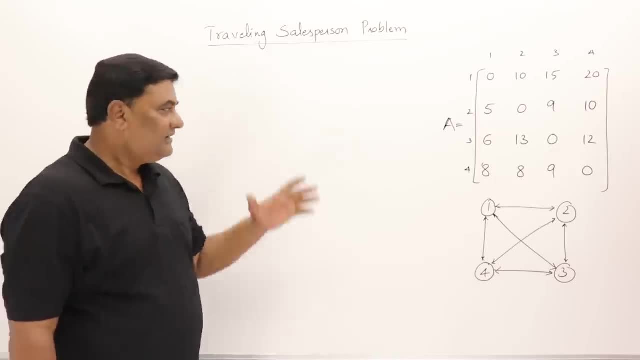 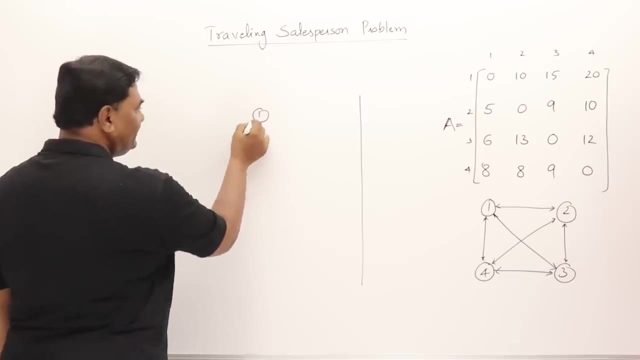 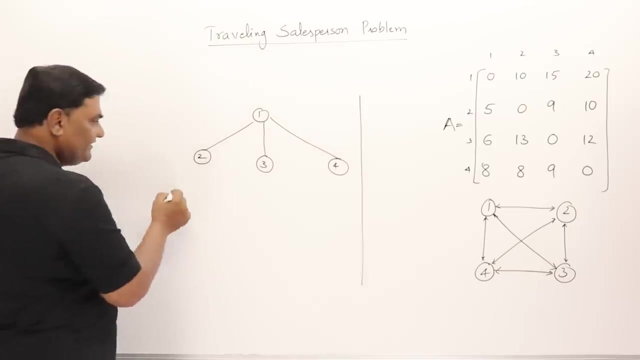 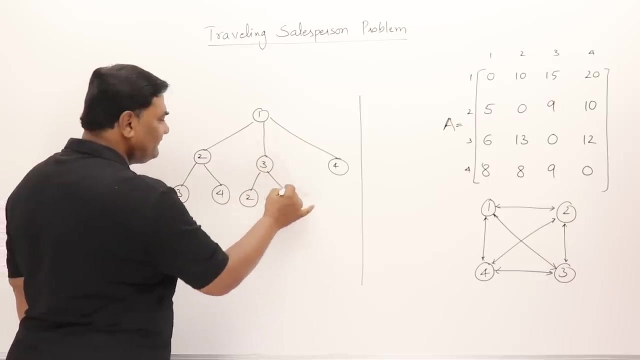 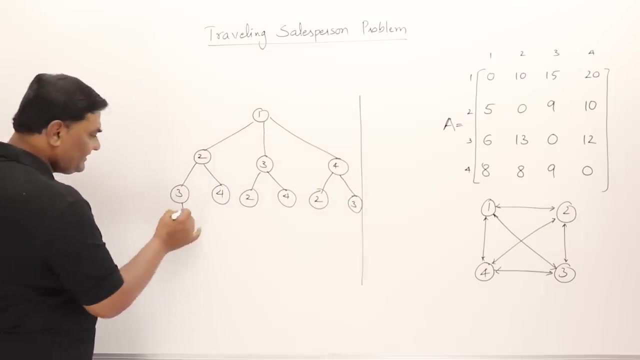 show you how dynamic programming makes it easy: menos and 4.. If I select 3, the other remaining are 2 and 4.. If 4, then other remaining are 2 and 3.. Then after 3 the remaining vertex will be 4. only Here the left over vertex is 3,. 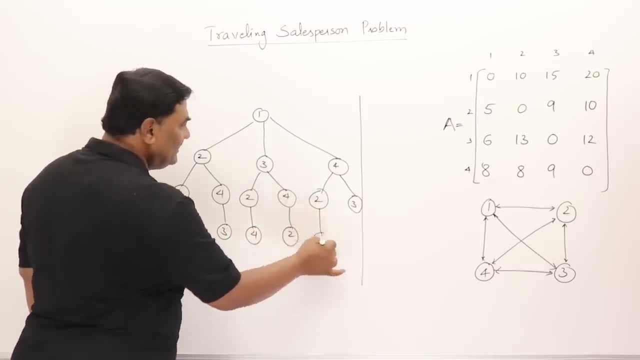 left over vertex is 4, left over vertex is 2, and that is 1, 4,. 2 is already over, so 3 is remaining. This is 1, 4, 3 is already over, so 2 is remaining. See, these are the possible. 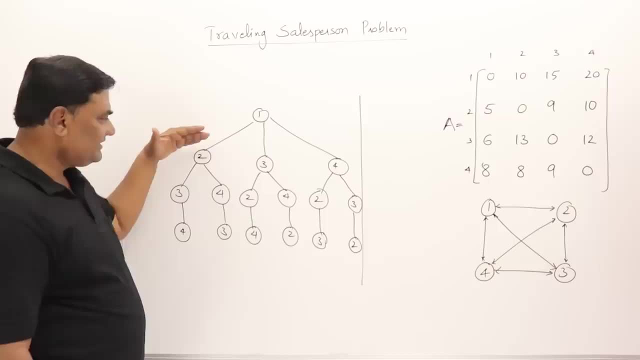 routes that a salesperson can take. He can start from 1, then he can go to 2.. He can start from 1, then go to 2, then 3, then 4, or 1 then 4, then 4, then 2, then 4, then 3.. 1,, 3,, 4, 2. 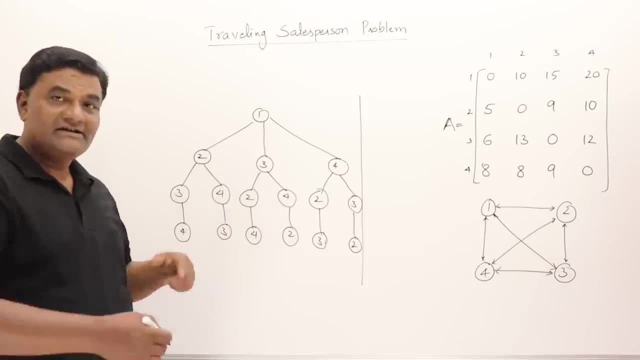 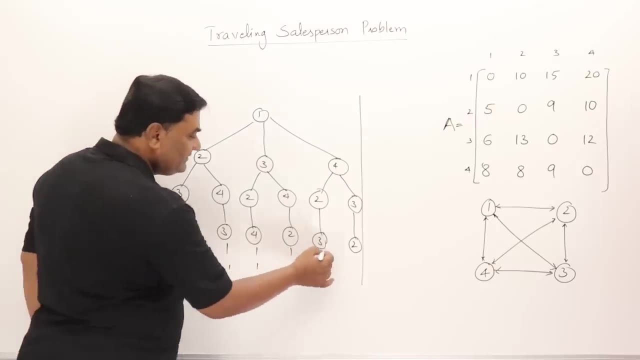 like this. There are many possible routes. Then after that he has to return back to starting vertex 1, only See. after 4 he has to come back to 1,, come back to 1,, come back to 1.. Right Now I should know the minimum cost route. 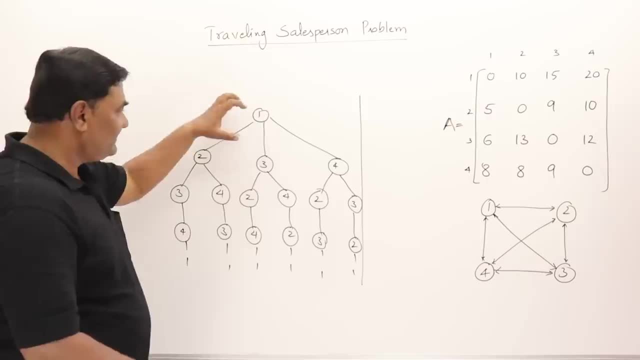 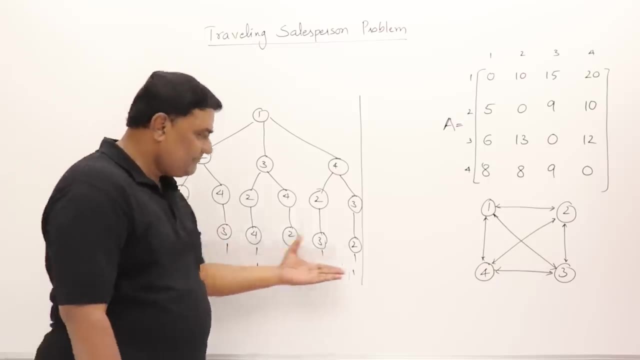 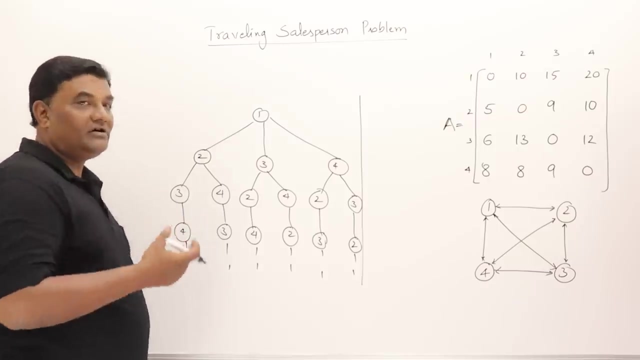 From starting vertex 1.. If I select this one, then I have to know the cost of all these, so the problem becomes very big. Let us start solving it from bottom. If he is on salesperson, is on 4th vertex, then what is the cost Where he has to go, remaining When he is on 4th? 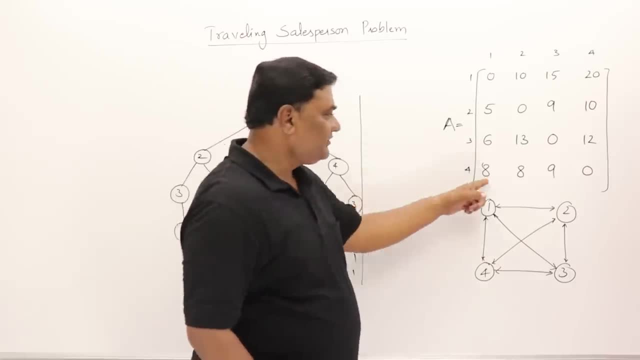 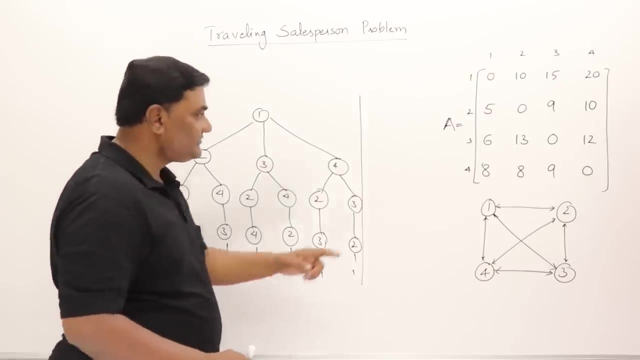 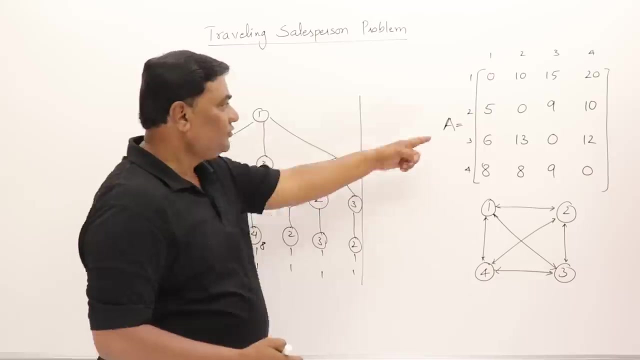 vertex, then he has to return back to vertex 1.. So vertex 1 cost is 8.. This is 8.. If he is on 3, what is the cost Of returning back to vertex 1.. 3 to 1 is 6, and this is 4.. Again, it is 8.. From 2,, 2 to 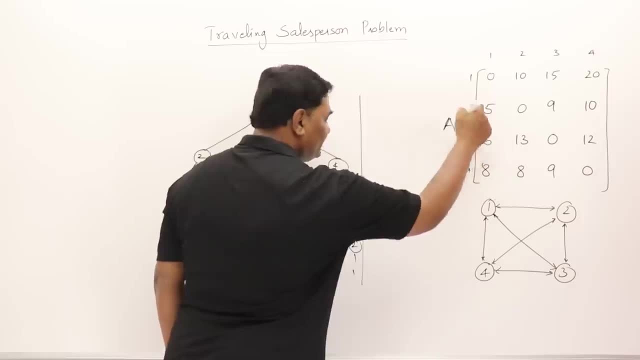 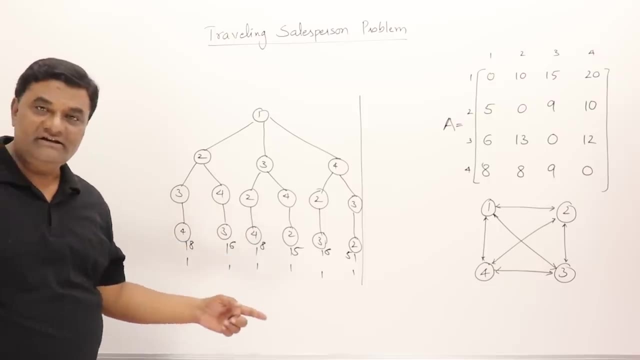 1 is how much? 5.. This one, Then 3 is already 6 and 2 is 5.. So I have written the cost here where he has to return back to the starting vertex 1.. Then if I say that he is on vertex 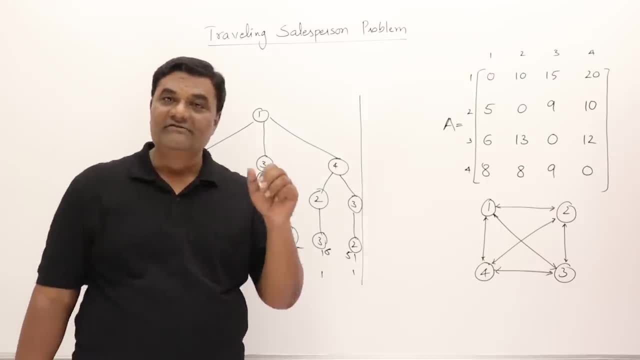 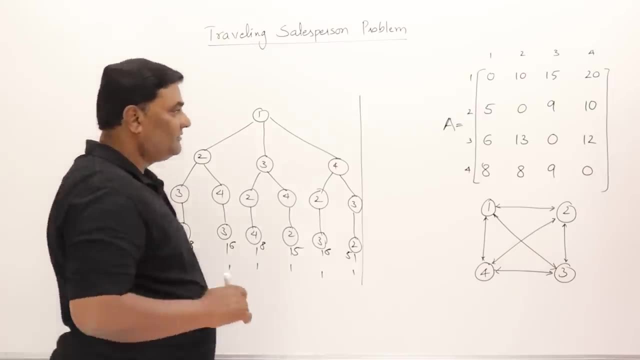 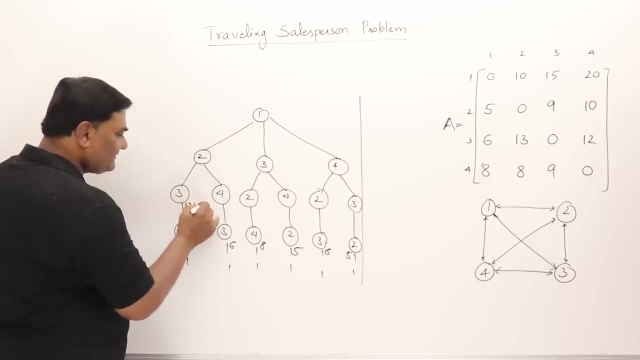 3. Then what is the cost? the cost of reaching the starting vertex from there. so from 3 he has to go to 4, then to vertex 1. so 3 to 4. how much? 3 to 4 is 12, 12 plus 8. this is 20 and he is on 4, he has to go on 3 and then. 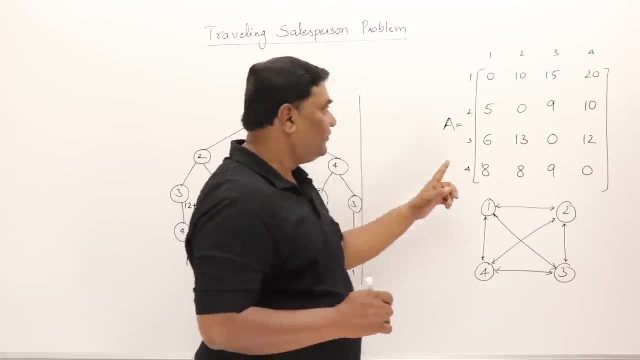 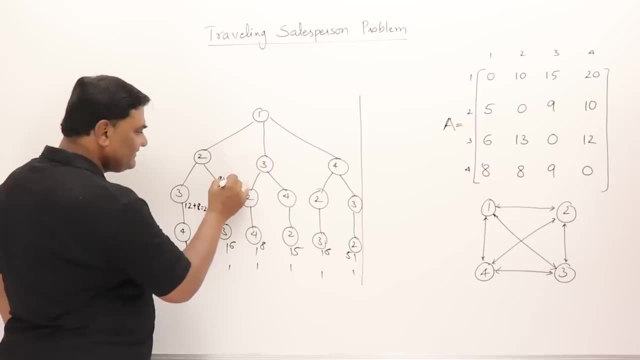 return back to vertex 1, so 4 to 3, how much? so 4 to 3 is 9 plus 6, so this is 9 plus 6, this is 15. now suppose he is on vertex 2 then, where he has to go next vertex 4 and then return what? to the? 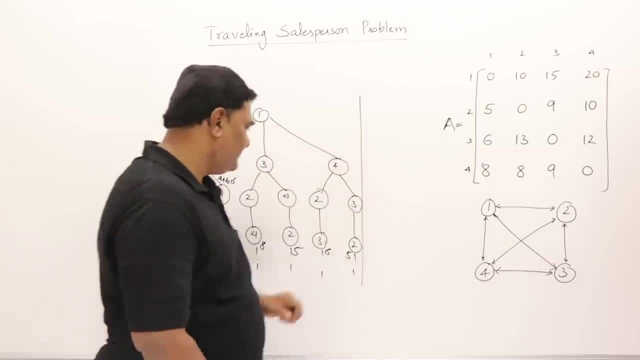 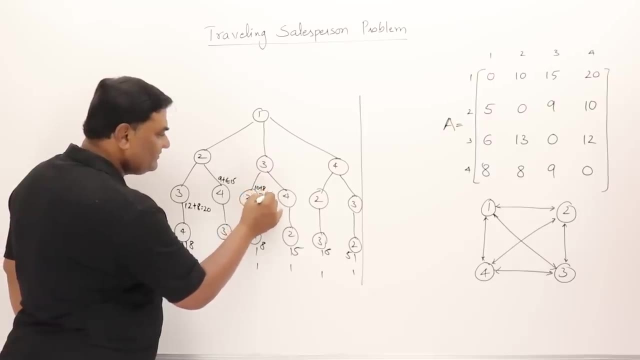 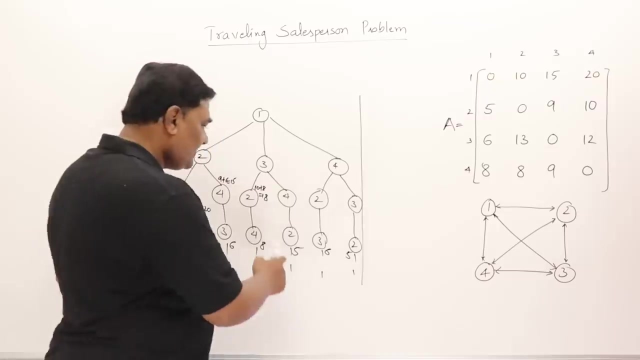 vertex 1. so 2 to 4. how much? 2 to 4 is 10, 10 plus 8. so this is 10 plus 8 is 18. he is on 4. he has to go to 2, then return back. so 4 to 2 is how much 8? 8 plus 5. so this is 8 plus 5. 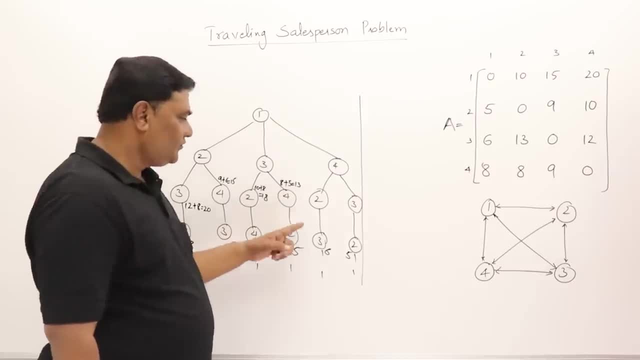 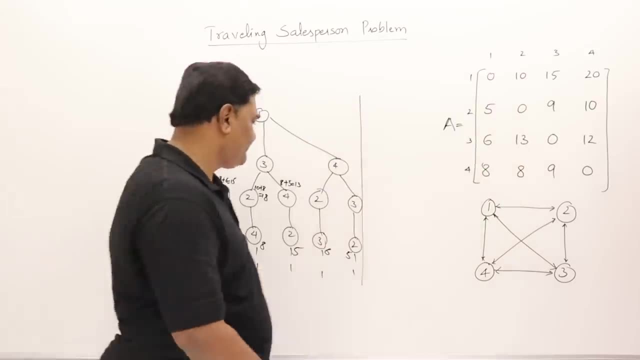 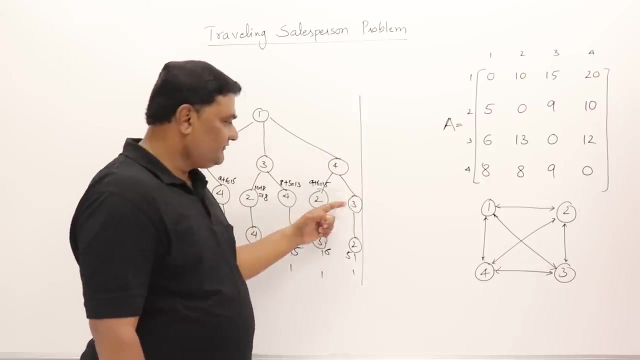 is 13. he is on 2. he has to go on vertex 3 and return back to vertex 1. so 2 to 3, how much? 2 to 3 is 9, 9 plus 6. so this is 9 plus 6 is 15, right? so he is on vertex 3. he has to return back to 2. 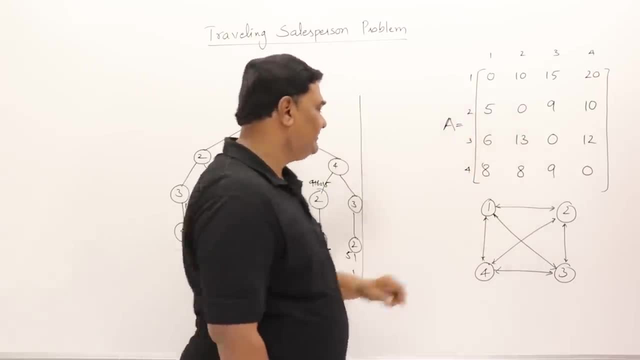 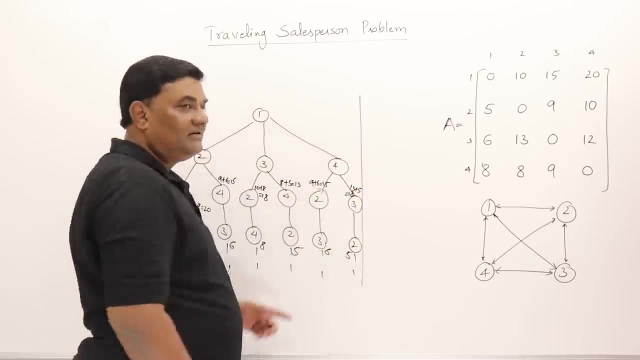 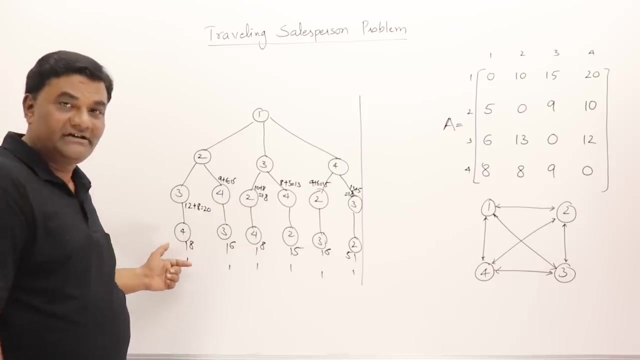 so 3 to 2? how much? 3 to 2 is 13, 13 plus 5. so 13 plus 5 is 18. so I started from the bottom. see, I am considering that he is on vertex 3 and remaining vertices are. he has to go on 4 and then return back to 1. now let 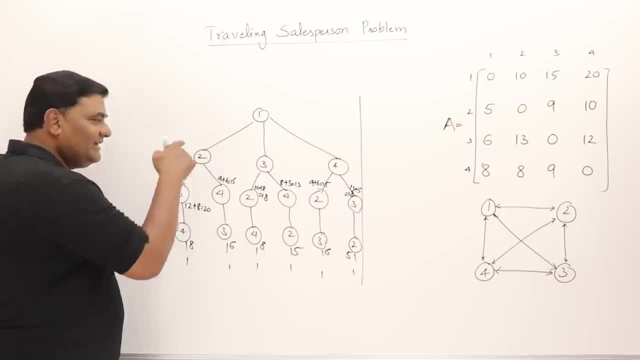 us go one more level up here. now where he is, he is on vertex 2. vertex 2, then what are the remaining vertices? 3 and 4? so either he can go to 3 then 4, or he can go to 4 then 3. I have to take. 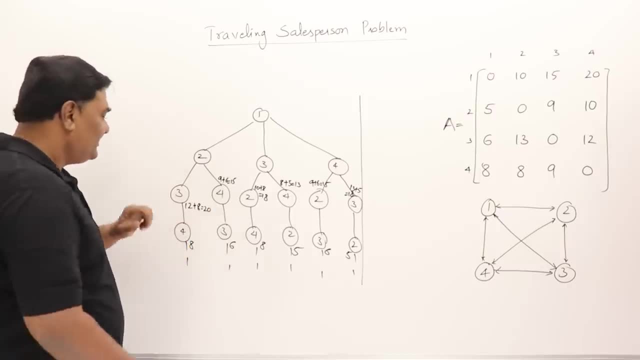 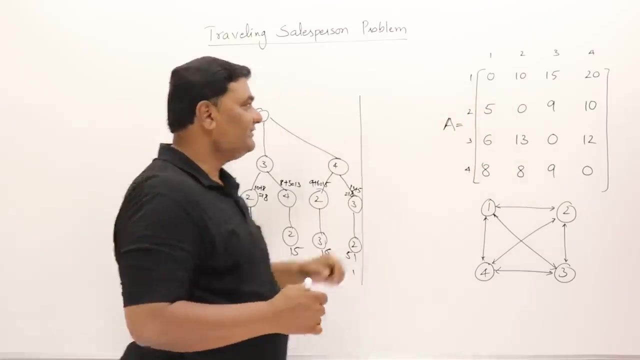 minimum out of these two minimum. so let us see 2 to 3: how much 2 to 3 is 9, so this is 9 plus how much it is 20. and 2 to 4: how much 2 to 4 is 10 plus how much. 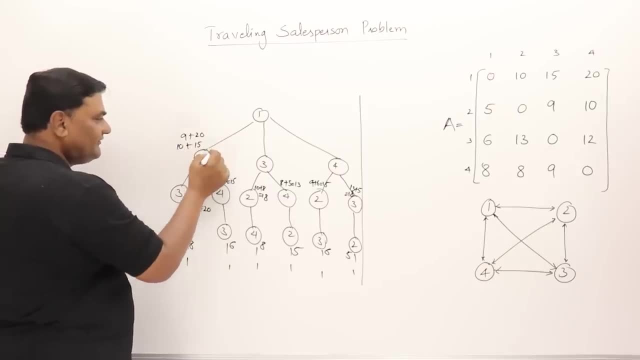 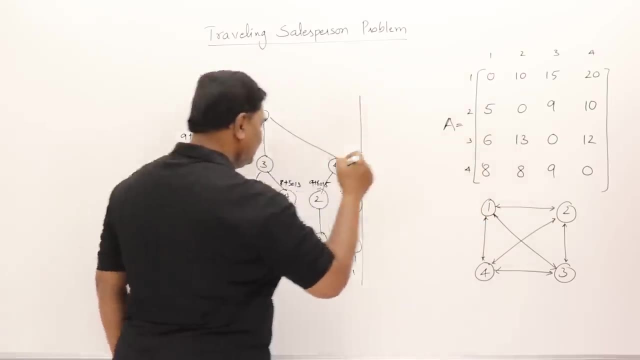 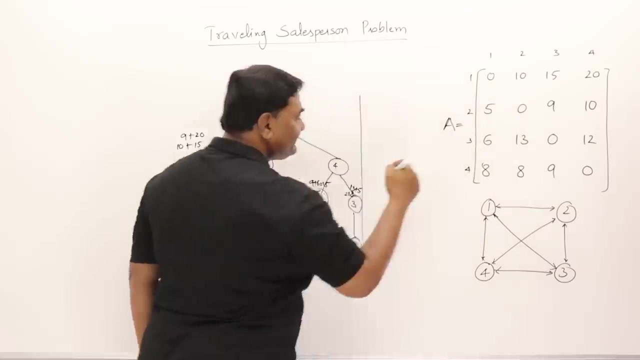 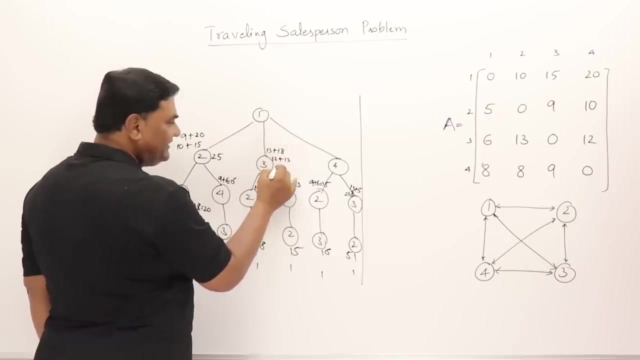 this is 15, which gives minimum result 25, so this is 25. now same way, 3 to 2, 3 to 2, 13 plus 18, and this is 3 to 4. 3 to 4 is 12 plus 13. now this is 31, and this is 25, so this is also 25. now 4. 4 to 2. how much. 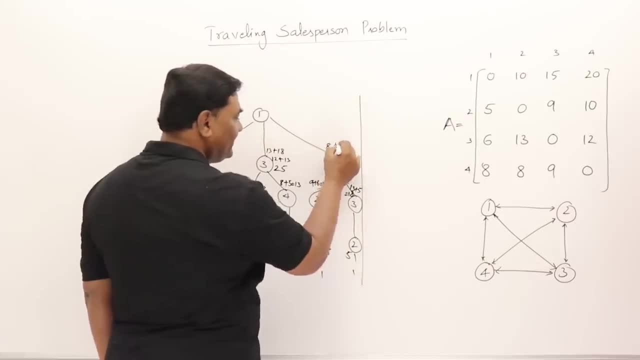 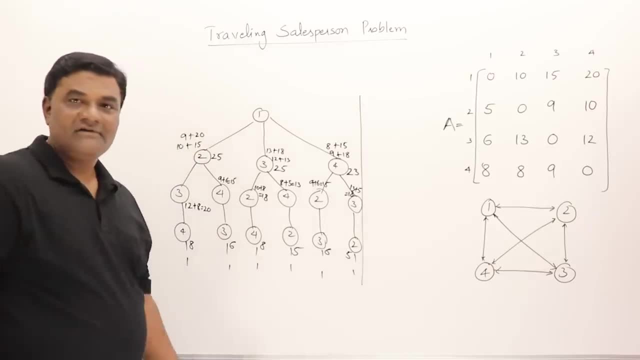 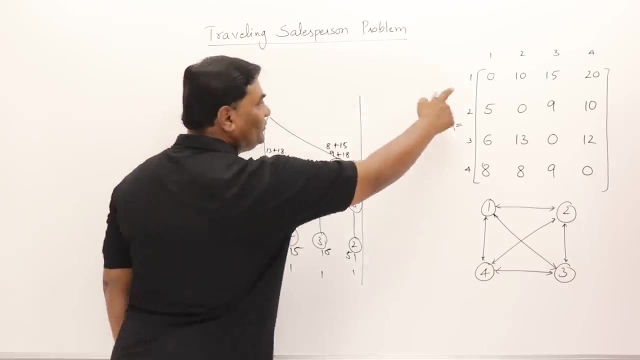 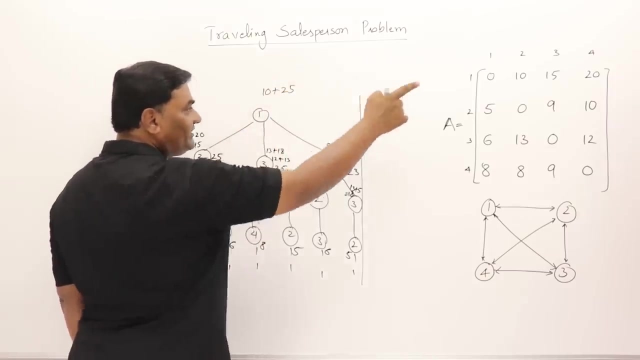 smaller. So this is 23.. Now I can know the cost of this one. What is this? 1 to 2.. 1 to 2 is how much? 10 plus the cost of this is 25.. And this is 1 to 3.. 1 to 3: how much? 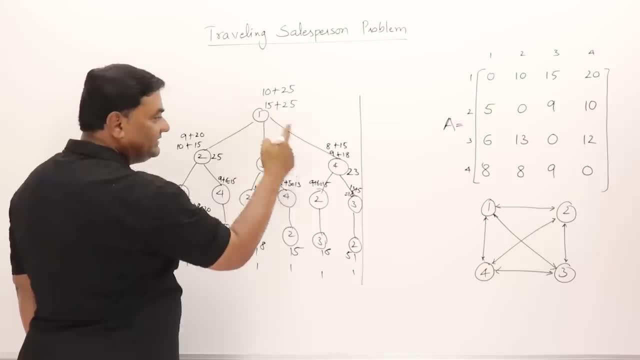 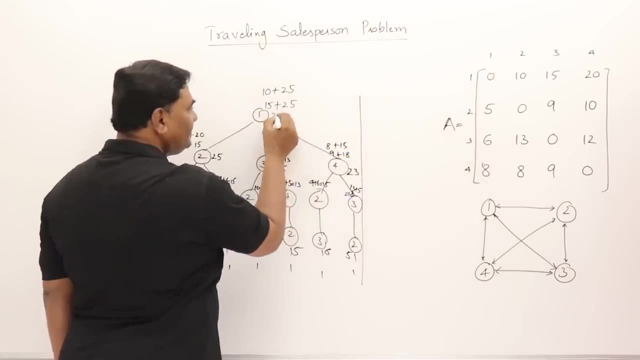 15 plus this is 25.. And 1 to 4 minimum, how much 23.. And 1 to 4 is how much 20.. 20 plus 23.. Out of this, which is minimum, This is 35,, 40,, 43. So this is 35.. 35 is minimum. 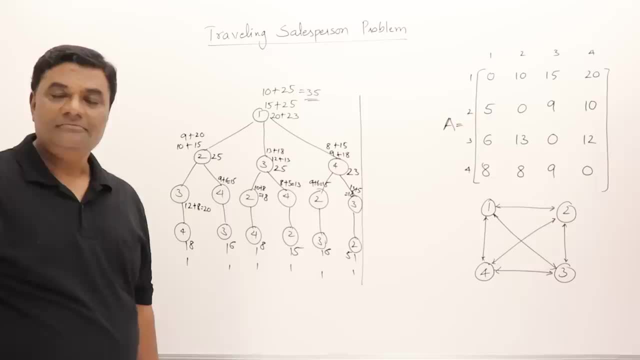 That's it. The cost of shortest route is 35.. I have shown it using brute force approach and I have written the cost here. Right, But let us see how dynamic programming works on this one. So from this we can get the idea about the formula and I will show you how. 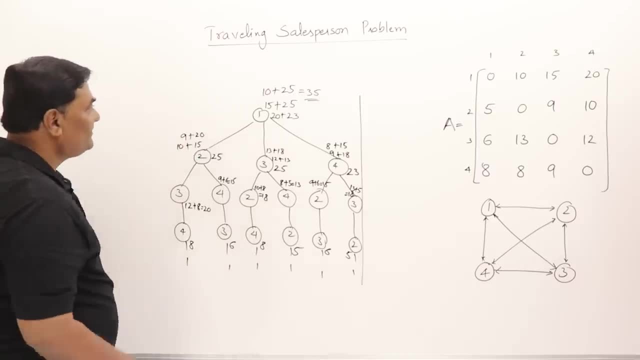 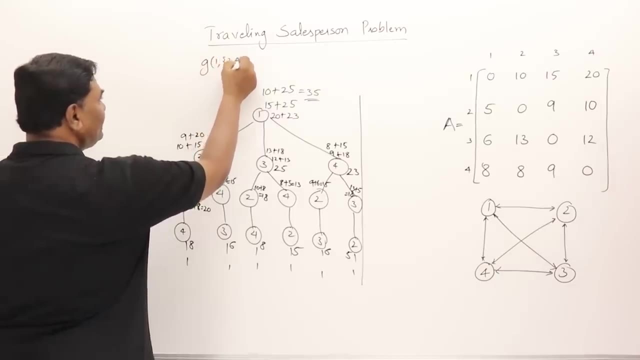 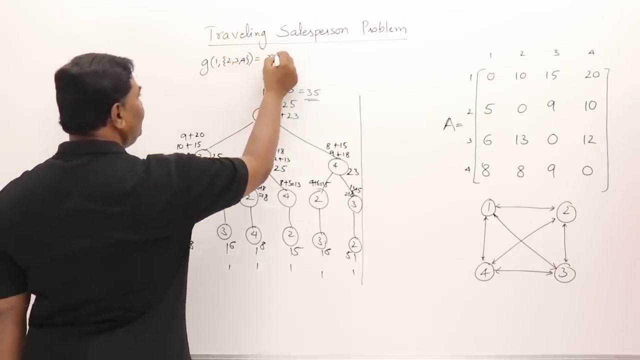 actually we solve it using dynamic programming. See, the formula is like this. The cost, if it is represented as the starting vertex, has 1 and the remaining vertices, that are that I have to visit, are 2, 3, 3 and 4.. Then I have to take minimum Right From 1 to 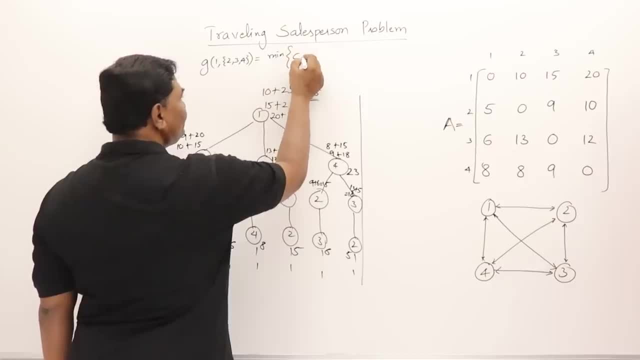 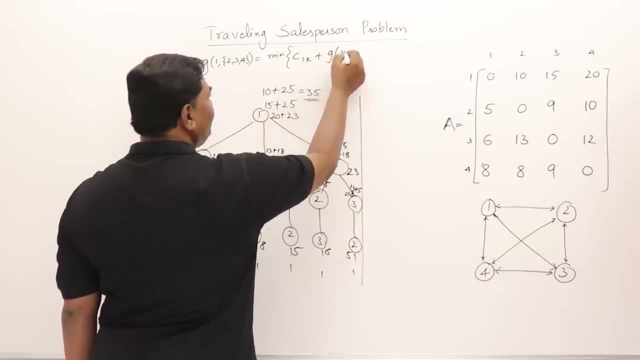 2, or 1 to 3, or 1 to 4.. So cost of an edge from 1 to any k, plus cost of from that k vertex, See 1 to 2.. So then k, 2 to remaining. If 1 to 3, then 3 to remaining. So 1 to k, k to 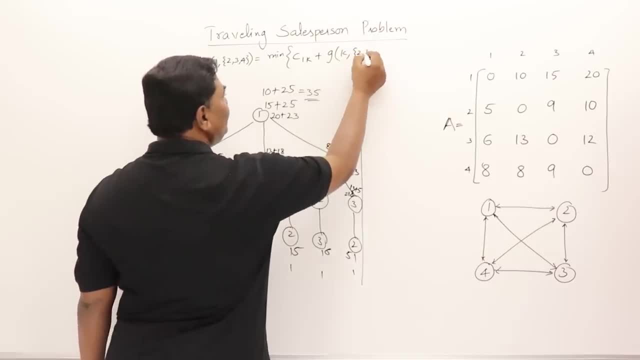 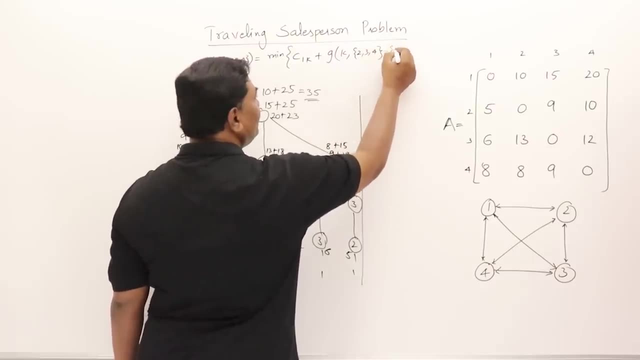 remaining Remaining is what? 2,, 3,, 4, with the vertices. Out of this, whichever one I have taken, I should subtract that one, So k. So this means that I should try for all the k values. So I should. 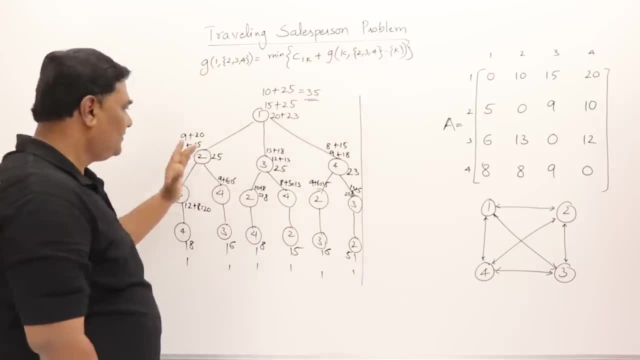 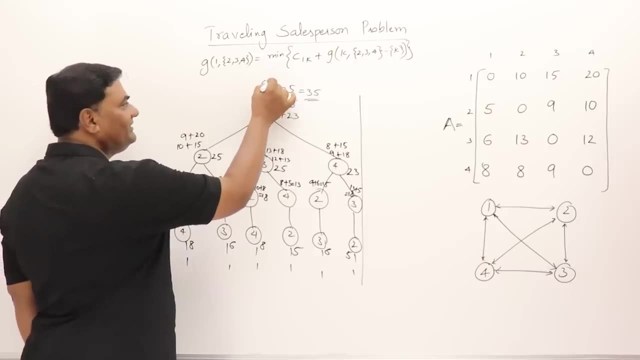 take the vertex as 2 also, 3 also, 4 also, So 2 also, 3 also, 4 also, Out of this, whichever is giving minimum that I have taken. So this is c of i k, Right c of 1, k And this is: 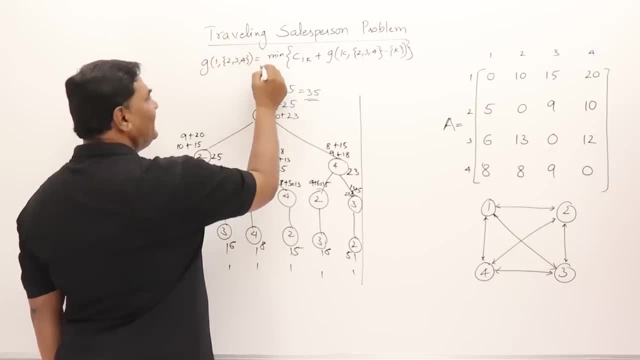 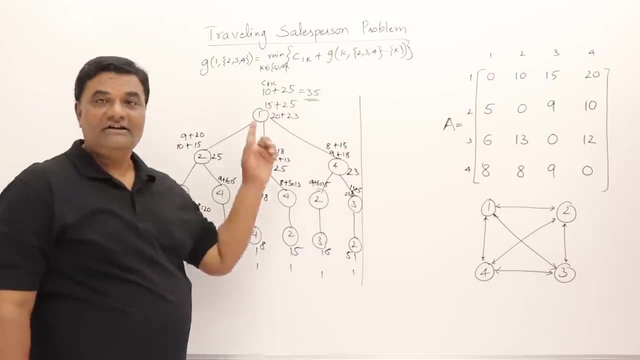 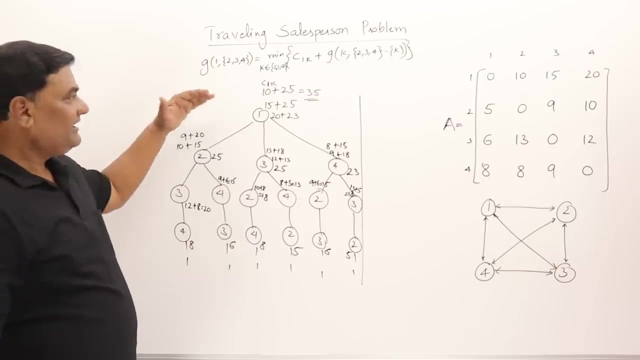 cost of remaining, and k takes the values. that belongs to 2,, 3 and 4.. This is the formula for one as a starting vertex. All right, And there are total 4 vertices. Now, if I write the general formula for this one, I will just remove this. If I write the general formula, g- cost of 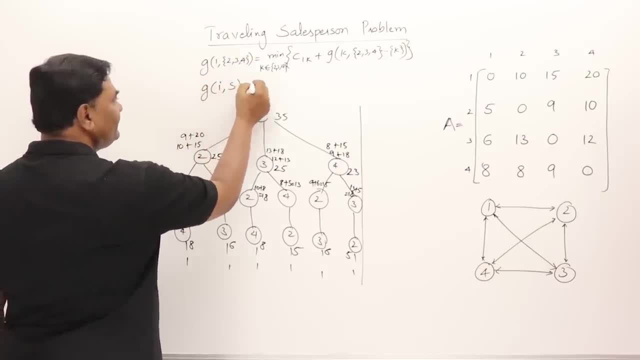 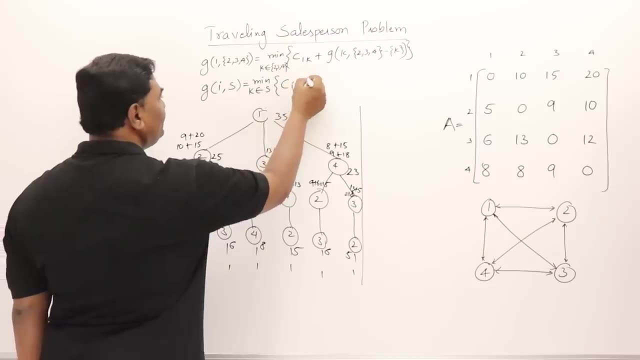 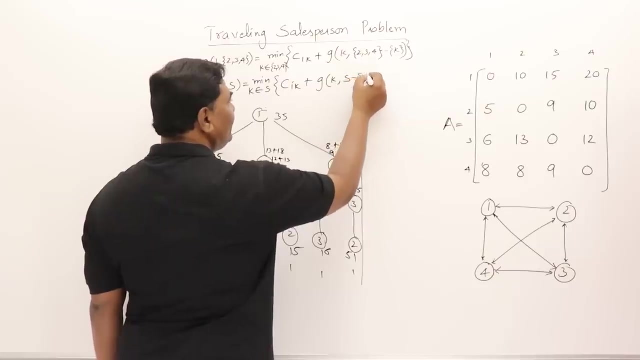 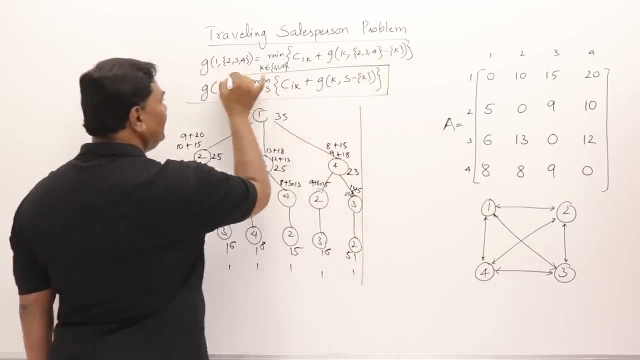 i some starting vertex, 2 set of vertices. Then minimum of k belongs to this set of vertices. this is c of i to k plus cost of k to set, and from this set I should subtract this kth vertex. this is the formula, this is the general formula that is followed by dynamic programming. so I 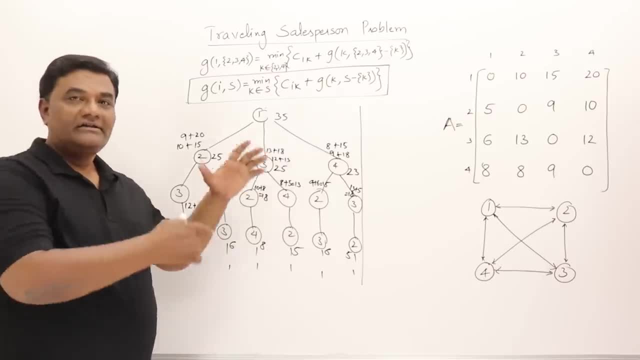 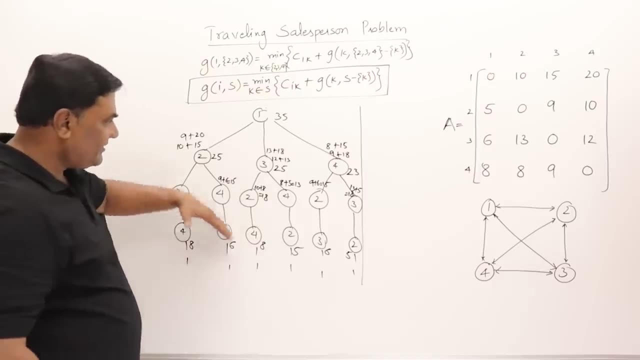 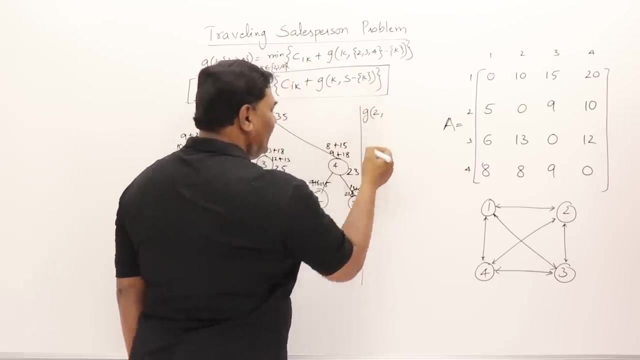 have shown you how the formula is derived. now, using this formula, how dynamic programming works. I'll show you, right see, as we have started solving from here, right. so first value that we'll find out is: let us say we are on vertex 2 and where we have to go next. we are on vertex 2. 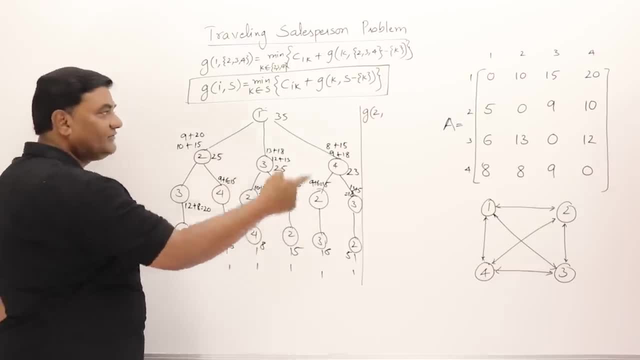 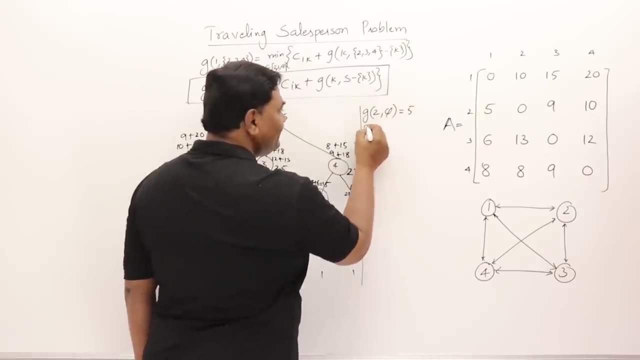 where we have to go, where next, nowhere. so nowhere means what we have to come back to vertex 1. so this is 5, nothing else. so what was this cost 5 then? similarly, if we are on third vertex and we have to return back to the first vertex, so third vertex, return back means 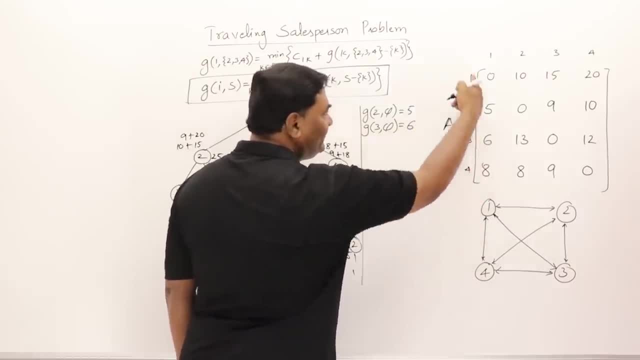 same thing. we have to return back to the first vertex, so third vertex, return back means same thing. we have to return back to the first vertex, so third vertex, return back means same thing. so from here on, so you can take: this is three two one, three two one, so this is three two one. 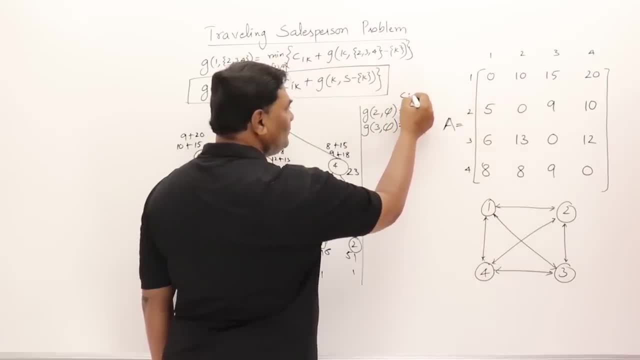 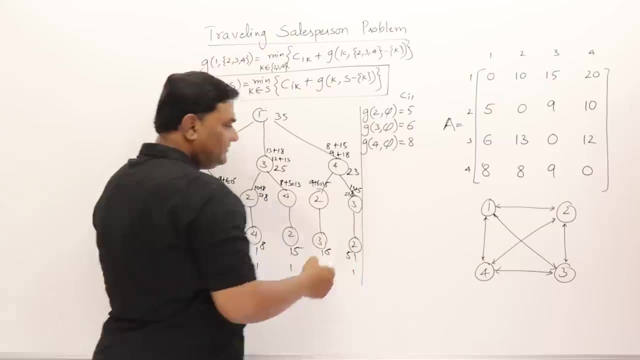 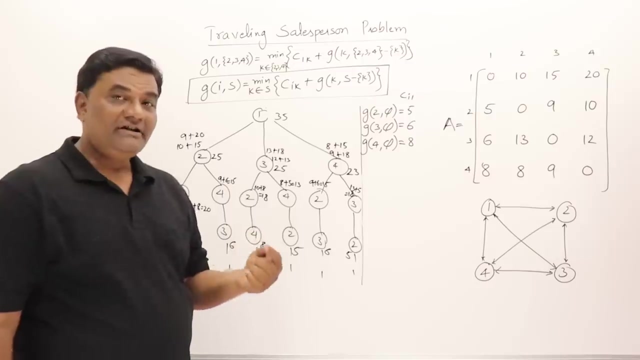 or this is c of whatever. I is to 1. right, then we are on fourth vertex and we have to written back to vertex one. so four comma one is eight. this is remaining vertex is nothing. now. next set we generate that. now we'll consider one vertex is remaining. what is that? see I? 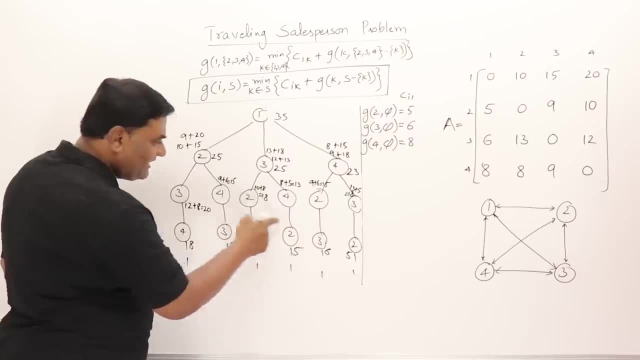 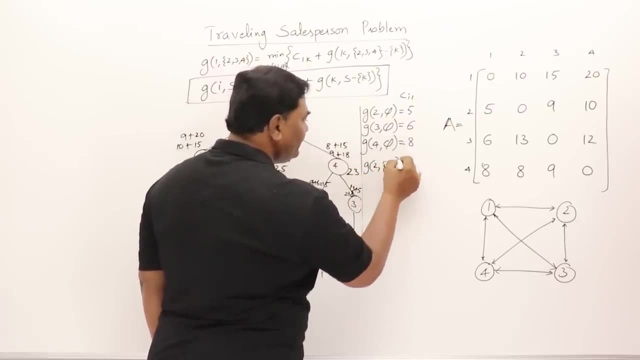 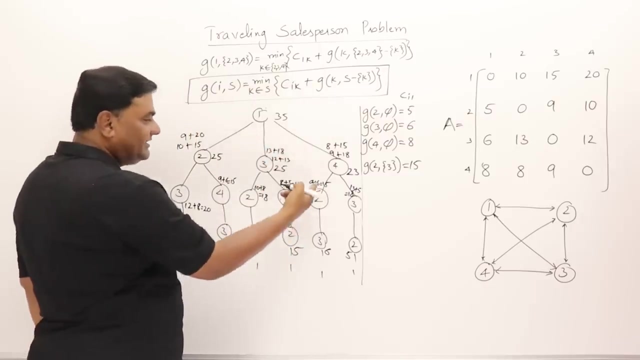 am on vertex 2 and the remaining vertex is 3, or am, Yes, am- on 2, remaining is 4, right? so g of 2, remaining vertex is 3. so what was this? 2 to 3, this was 15 already. we found out this one right formula. if you apply the formula, the same thing happens. 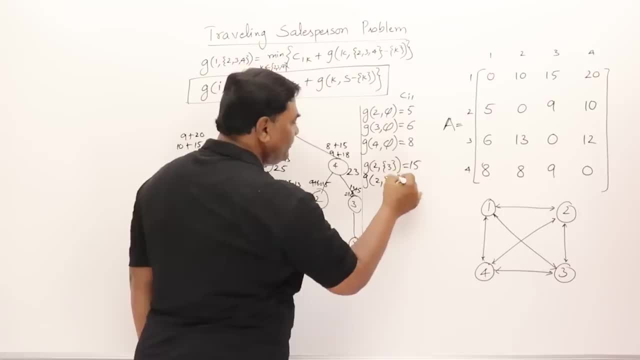 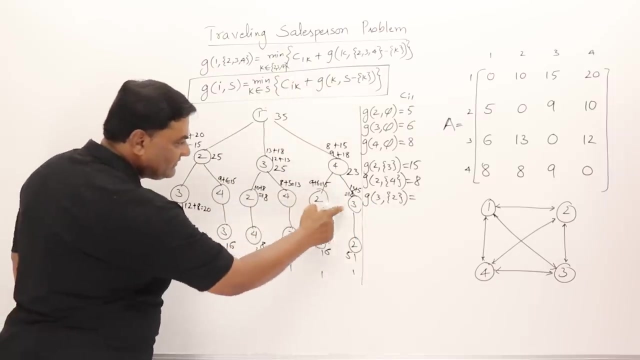 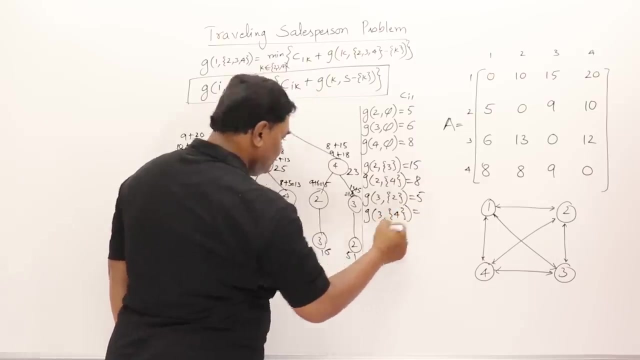 then am on vertex 2 and the remaining vertex is 4. so am on vertex 2 and the remaining vertex is 4. that is 8, and third vertex remaining vertex is 2. third vertex right. remaining vertex is 2. here 3 to 2, that is 5. third vertex remaining vertex is 4. third vertex remaining vertex is 4. 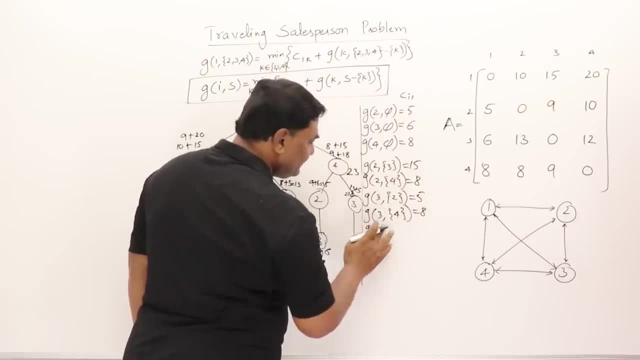 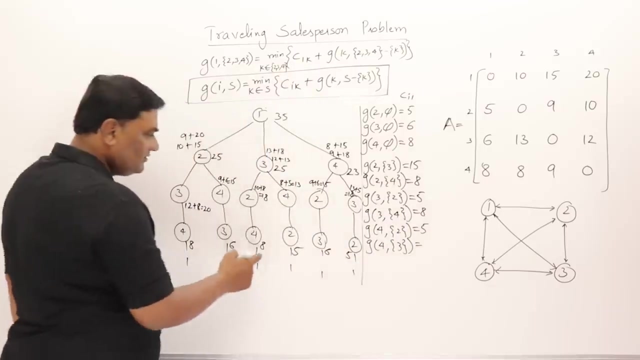 8, third vertex. fourth vertex remaining vertex is 2, 4 to 2. 4 to 2, 4 to 2 as a 5. 4th vertex remaining vertex is 3, 4th vertex, and the remaining vertex is 3, that is, 6. 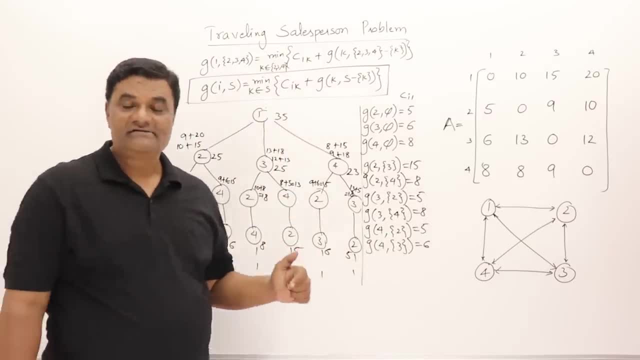 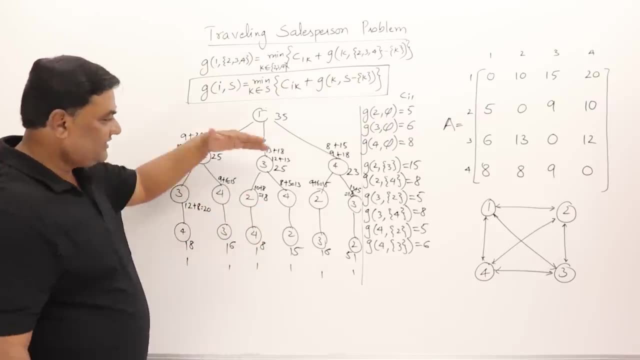 so we have considered that we are on some vertex and remaining vertex that we have to visit is only 1. now we have to consider: 2 vertices are remaining, so we are moving one level up. so we are on 2. remaining are these 2. we are on 3 and remaining are 2 and 4. 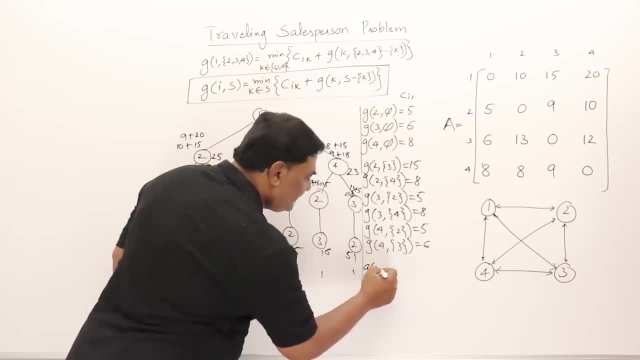 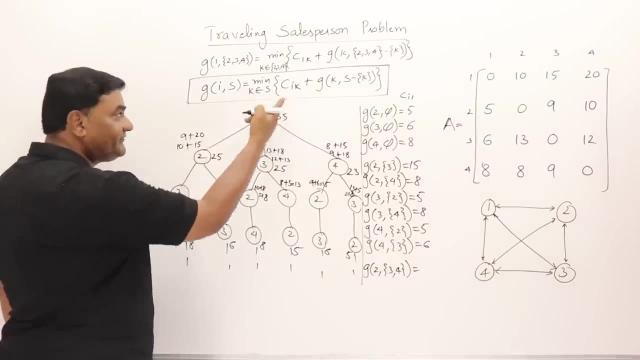 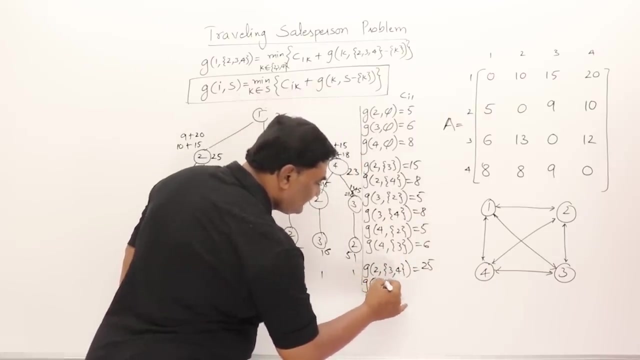 so for this we will prepare sets. we are on vertex 2 and the remaining vertices are 3 and 4 and the cost already we have found out minimum of these, 2 by using this formula only we were using, so this is 25 and g of third vertex. remaining vertices are 2 and 4. 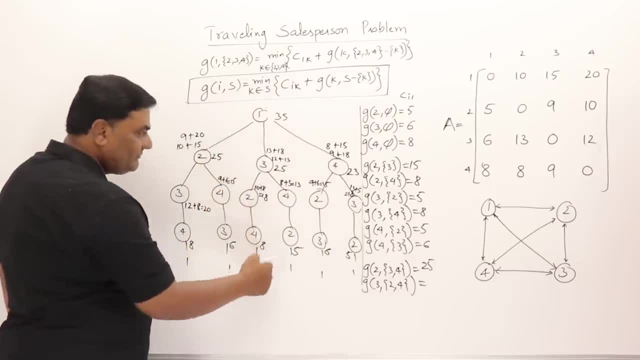 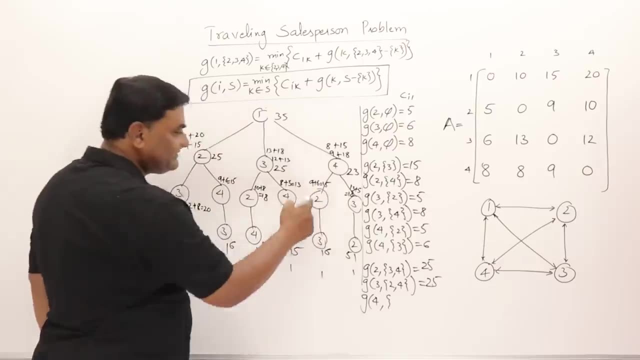 and we are on third vertex 2 and 4 remaining- we have to visit and the cost is 25. now we are on vertex 4. remaining vertices are 2 and 3, so this is 2 and 3 and the cost- already we have found out that- was 23. 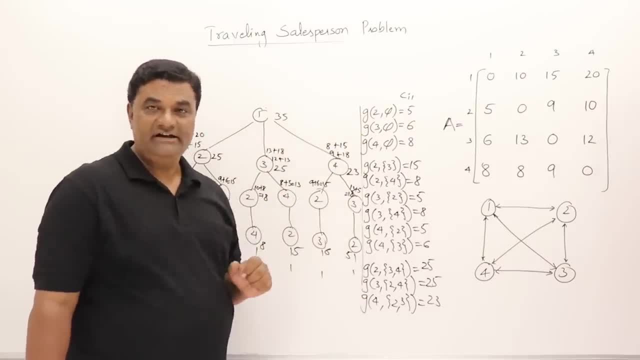 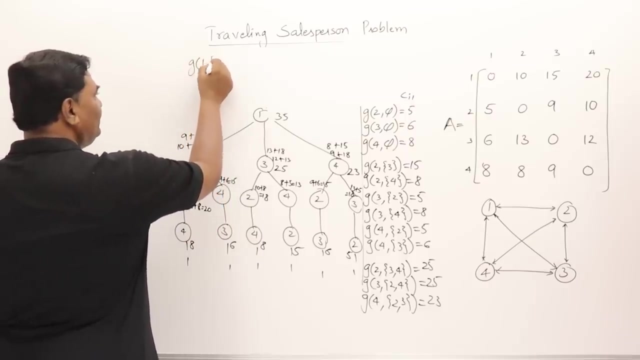 so, like a tabular values, I have all the values right. so already I have shown it using tree, but it is not solved using tree. it is solved like this. now, the last value that is remaining is: I am on vertex 1, g1, and the remaining vertices are 2, 3 and 4. 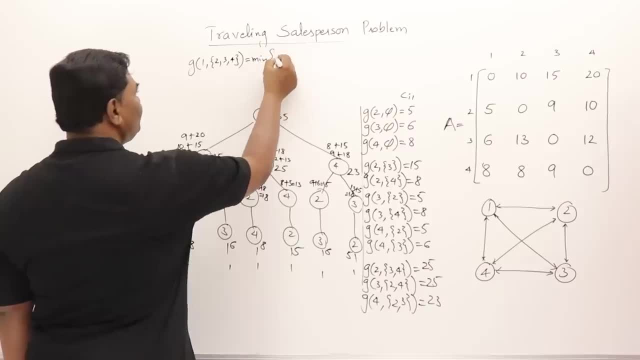 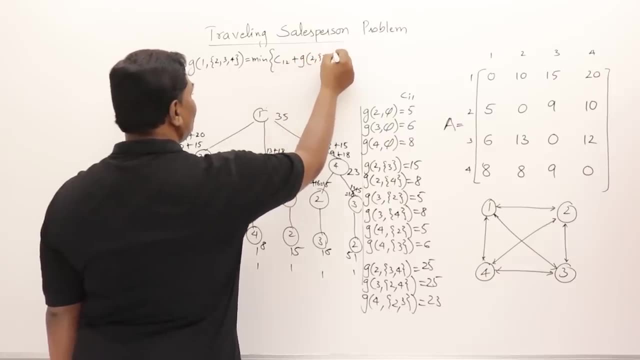 this is minimum of what? c of 1 to 2, plus g of 2 to 3, 4. right, I will use the formula instead of directly getting the answer: 35? we know already the answer is 35. then, instead of vertex 2, I will go on vertex 3. 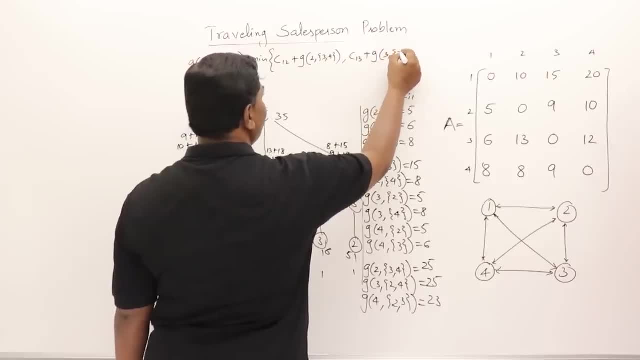 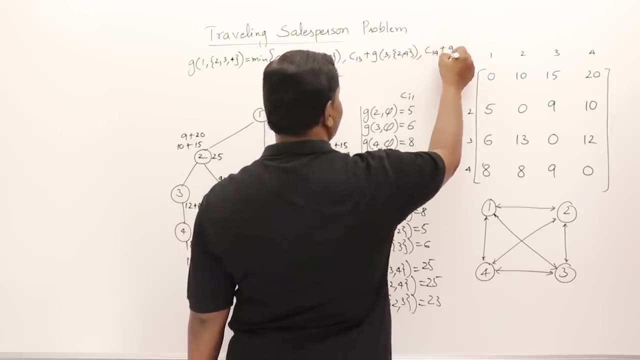 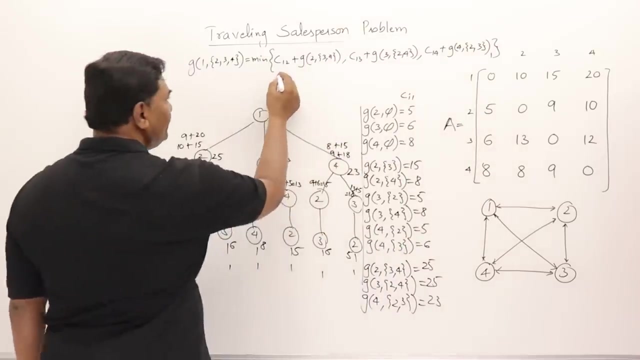 then this will be g of third vertex to remaining vertices that are 2 and 4, or I will go on vertex 4. then the remaining vertices are 4 to 2 and 3. out of this, which is minimum, see 1 to 2. 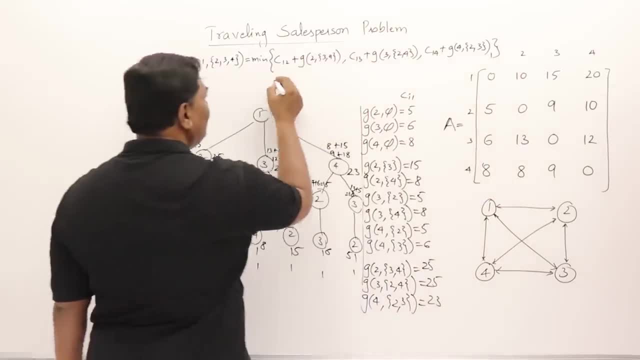 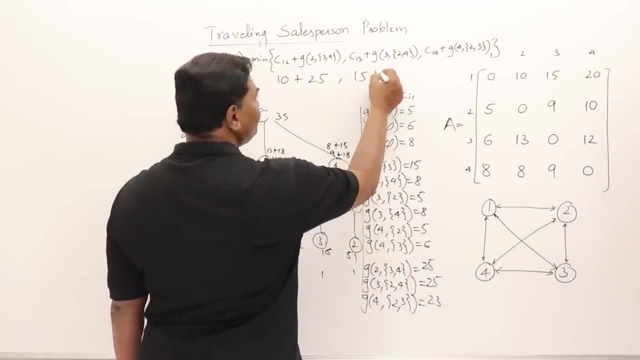 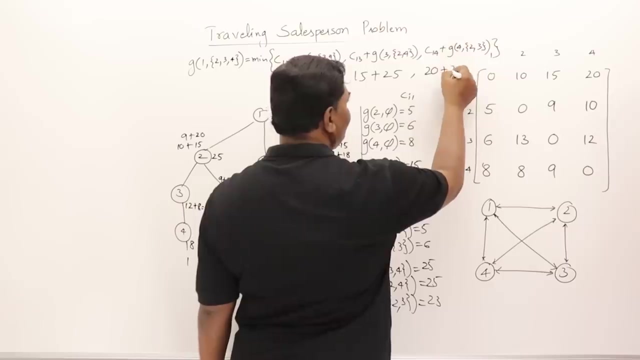 see 1 to 2,, 1 to 3,, 1 to 4 I need. so this is 10, 10 plus this was 25 here. I already have this. then this is 15 plus 25. then last one is: this is 20 plus 23. 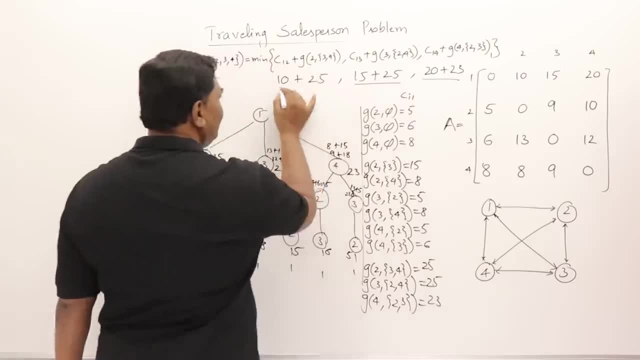 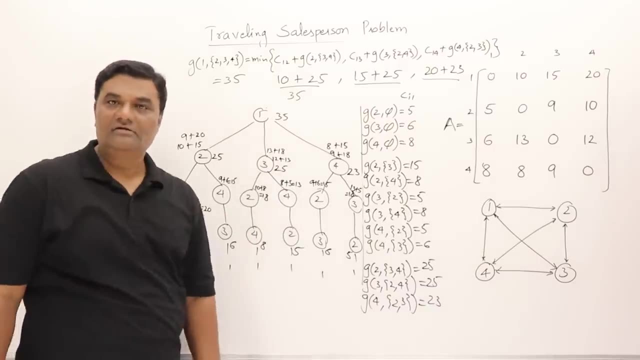 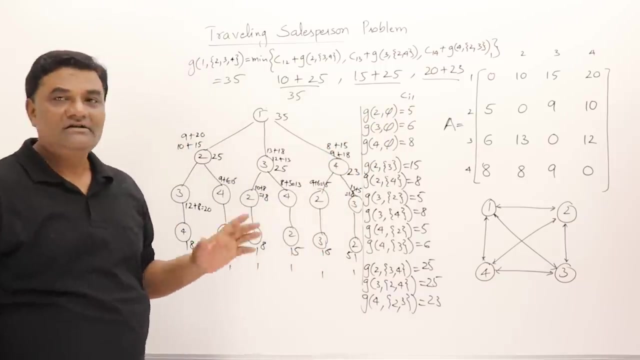 so this is 43 and this is 40 and this is 35. so, yes, the answer is 35, right? so if you prepare these values, you, by using the formula, you can get the answer. this is how travelling sales person problem is working. so what is the minimum path? 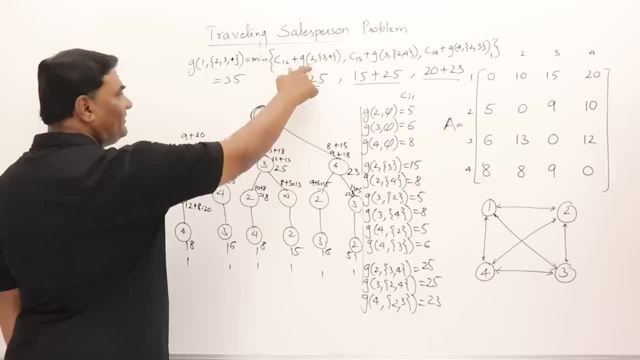 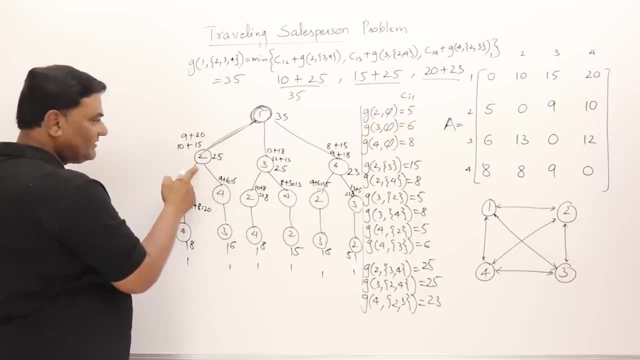 see, this is 35. because of what we got this as 35, we selected 2nd vertex as 25. this one right: 25 plus 10, 35. then this: we got a minimum from what 25? we got this one from this right. 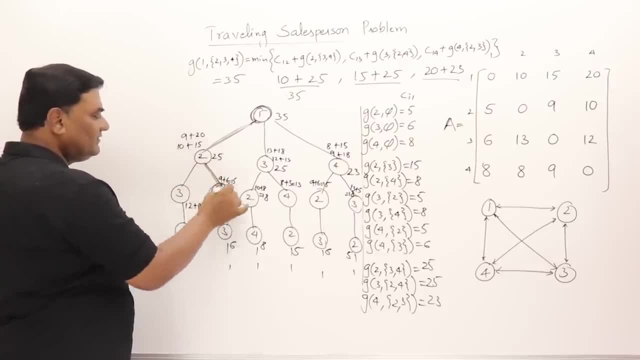 10 plus 15, 15. is this one right? so this one right. and then this- we got it from here- and this one, so answer is 1 to 2 to 4, then 3 right. so if you remember from which value are getting, 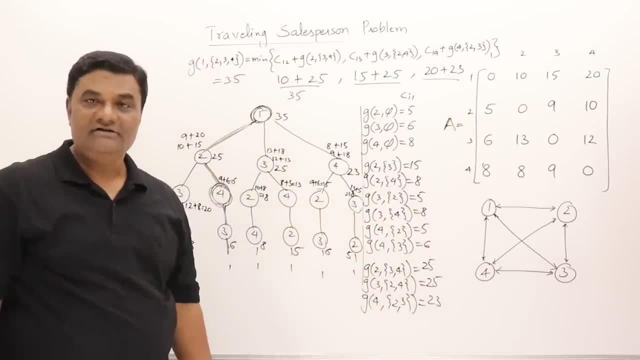 this minimum values, then from that also you can get the answer. so finally, we will solve the problem by taking sequence of decisions: where we will go next and we'll solve the problem. that's all about traveling salesperson problem. 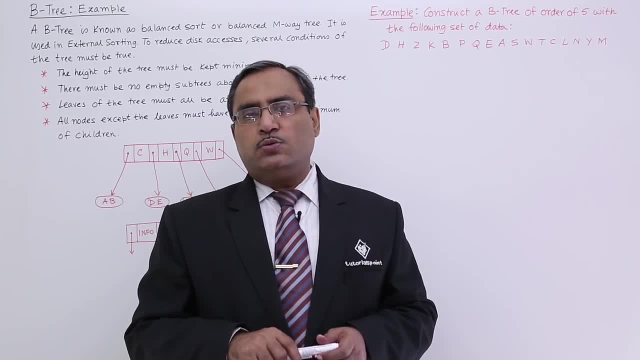 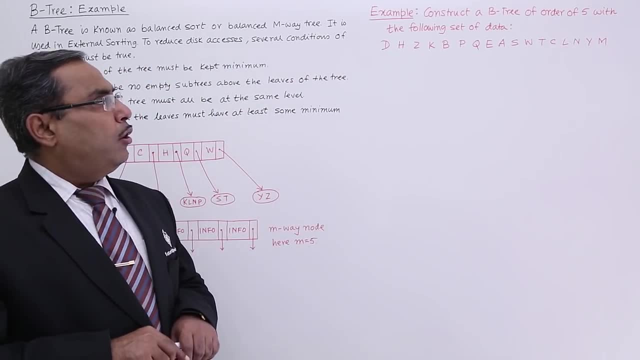 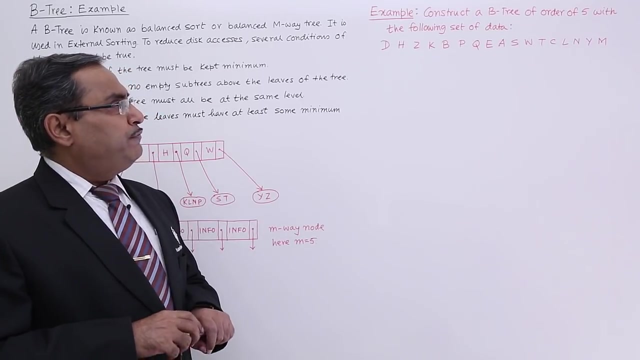 For the better understanding, let us discuss one example on this B-tree. So this is the example: Construct a B-tree of order of 5,, that means MOE B-tree. here value of M is equal to 5, with the following set of data: As it is of the order of 5, that means node will have the shape. 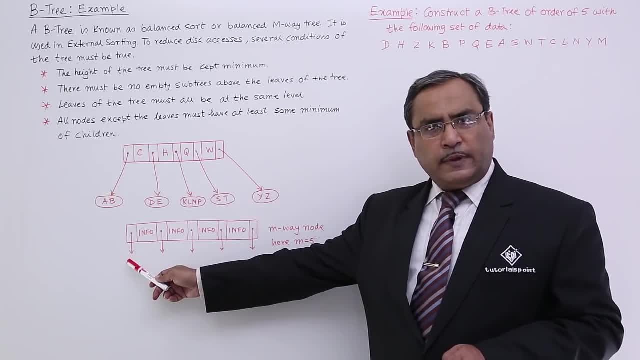 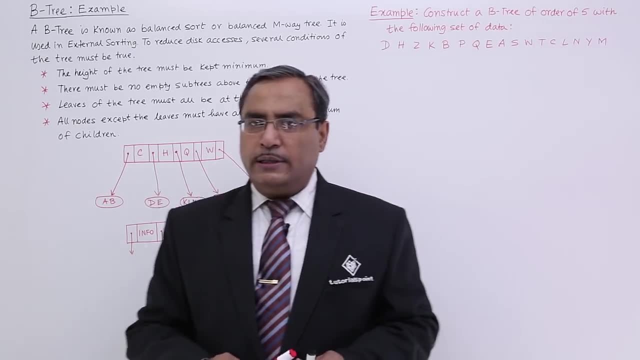 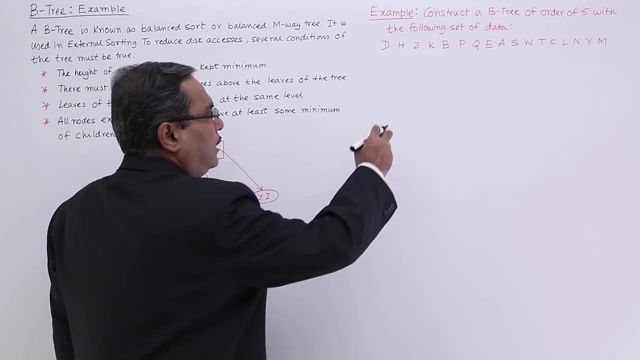 like this: that means 5 link fields and 5 minus 1, 4 info fields will be there. So, considering this one, we will be constructing the B-tree, So we are having this particular node. that means each and every node can hold maximum 4 data, So I am just taking one node here. So D will be coming. 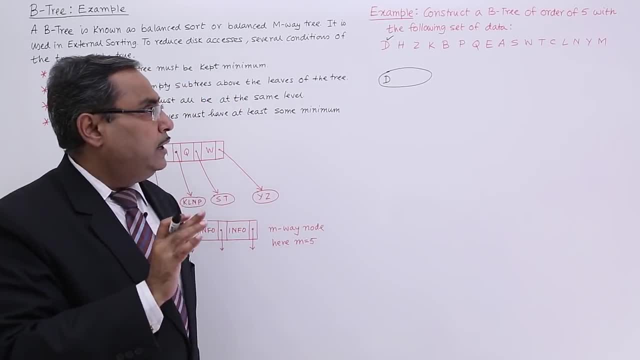 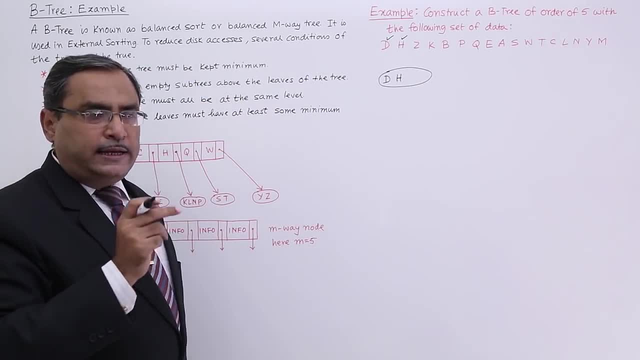 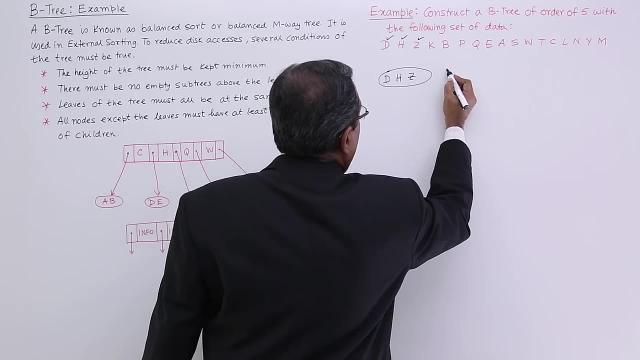 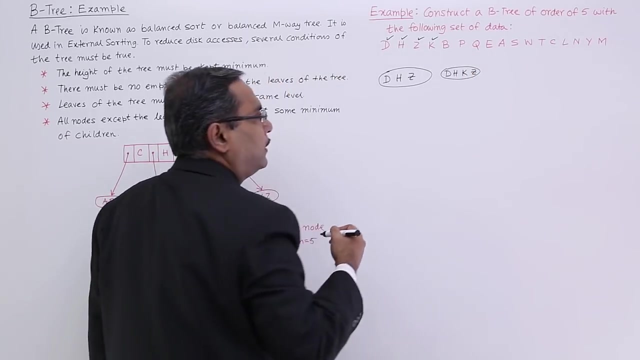 So H will be coming, Then Z will be greater than H, So Z will be coming and K will be coming before Z. So what will happen? So D, H, K and Z. So up to this we have done. Now you see, B will. 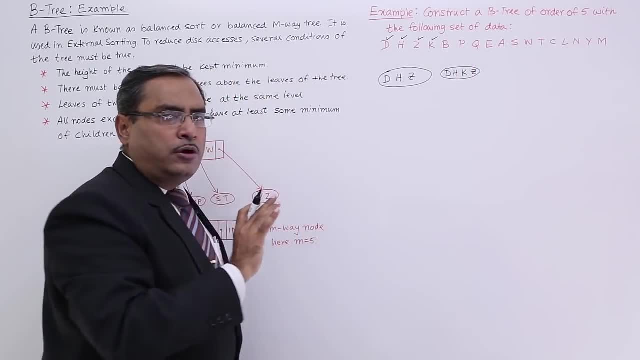 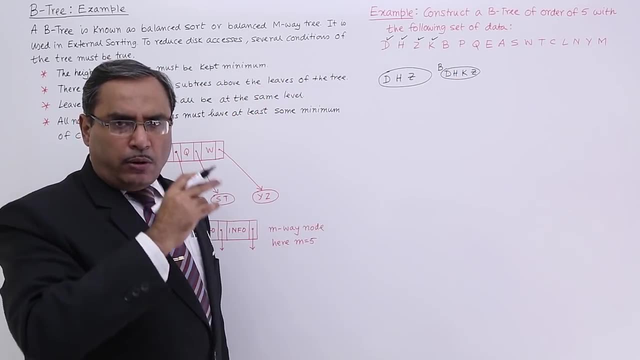 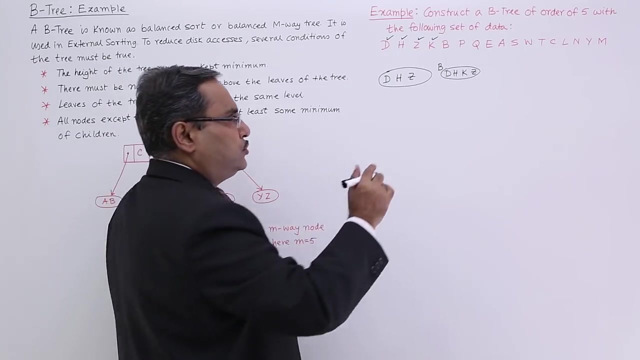 be coming. B cannot be inserted because it has already got 4 info. But if B got inserted then it will be before D. So now let me calculate the median. Median means middle, most data of the shorted data. So if you 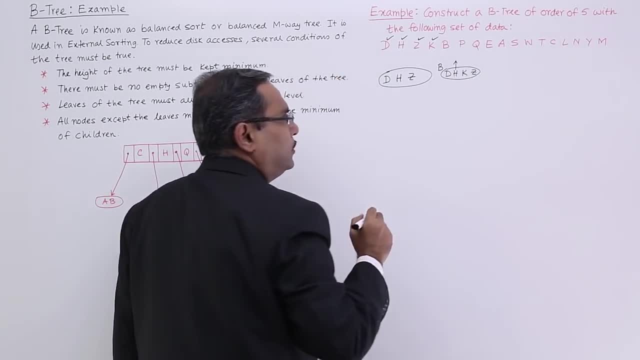 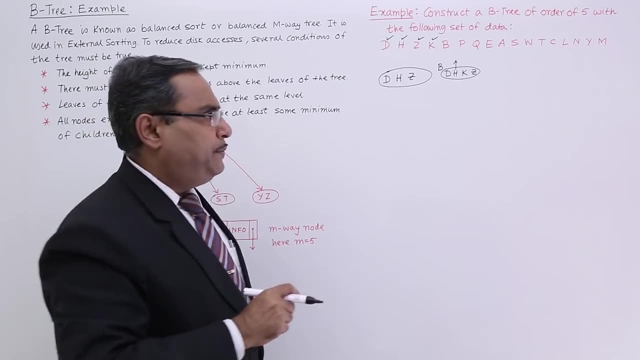 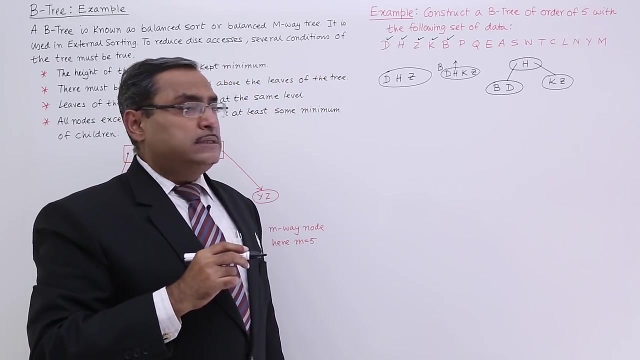 consider this one, then the middle most data will be H. So H is the median. So the node will split and H will contribute to its parent parent node C. So the B has got inserted. H was the median.